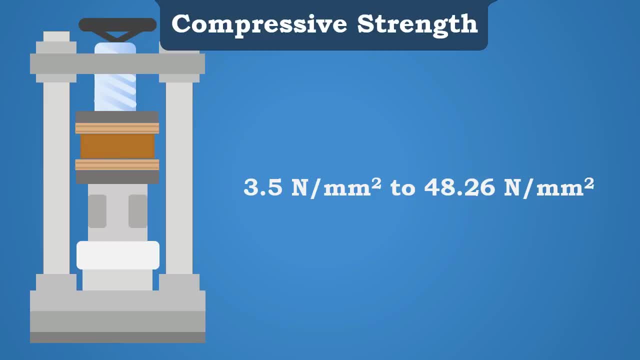 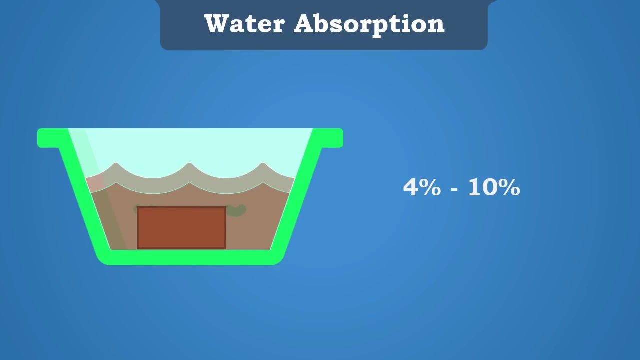 The compressive strength of fire clay bricks varies between 3% to 4%. These bricks are made of 2.5 N per mm2 and 48.26 N per mm2.. The water absorption percentage of fire bricks varies from 4% to 10%. 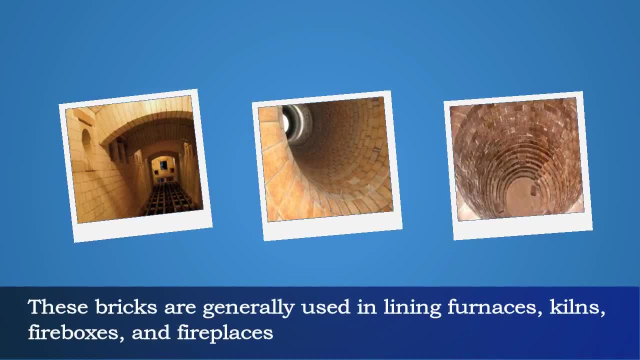 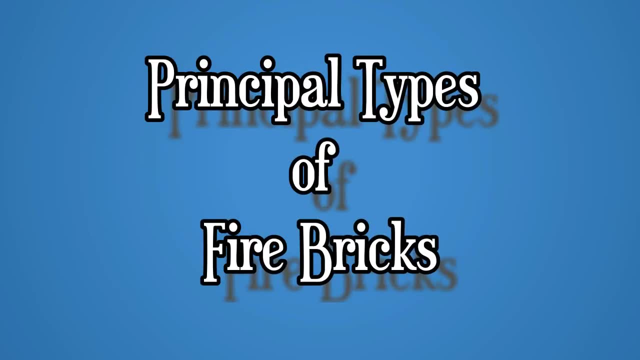 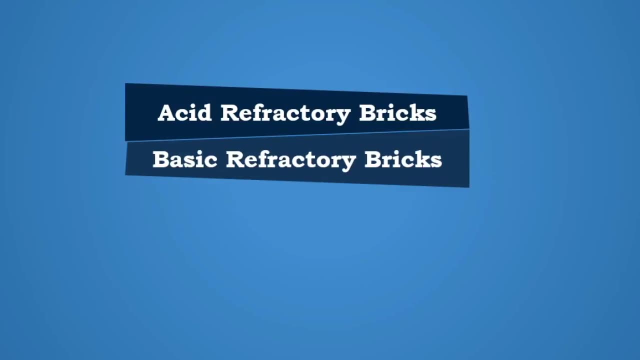 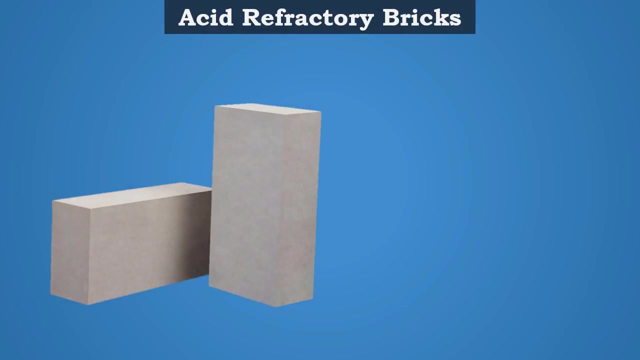 These bricks are generally used in lining furnaces, kilns, fire boxes and fireplaces. The principal types of fire bricks are Acid refractory bricks, Basic refractory bricks and Neutral refractory bricks. Acid refractory bricks are of two varieties. they are silica bricks and gannister bricks. 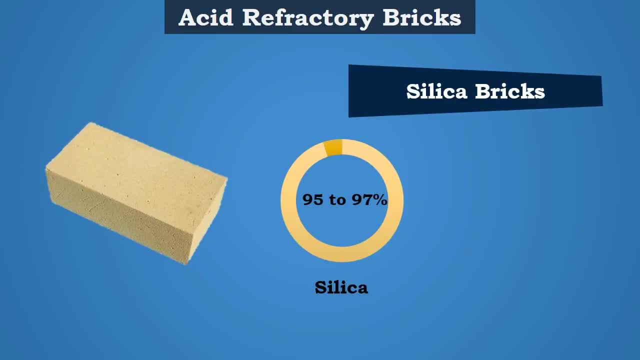 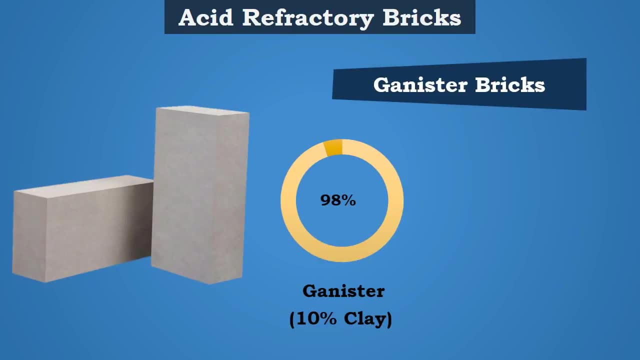 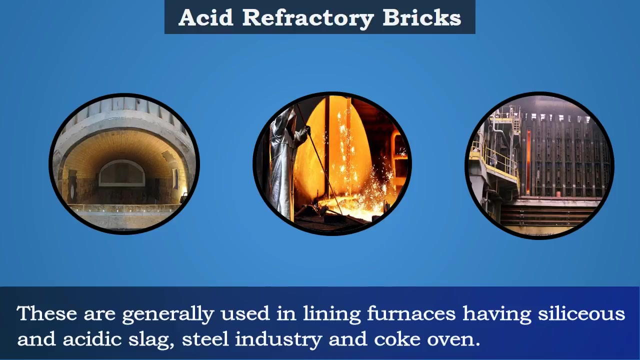 Silica bricks consist of 95% to 97% silica and 1% to 2% lime. Gannister bricks consist of 98% conister or hard colored stone with 10% conister. These are generally used in lining furnaces having siliceous and acidic slag, steel industry and coke oven. 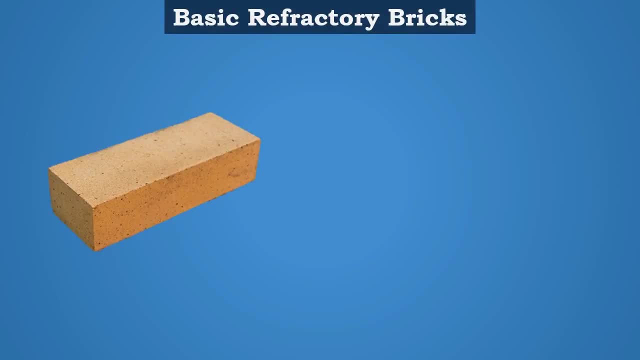 Basic refractory bricks. Basic refractory bricks are manufactured from magnesia, dolomite, bauxite, etc. The common two varieties are magnesia bricks and bauxite bricks. Magnesia bricks consist of magnesia above 85%, calcium oxide up to 25% and silica up to 5.5%. 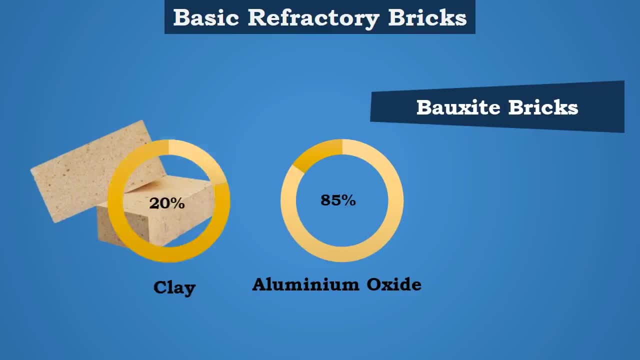 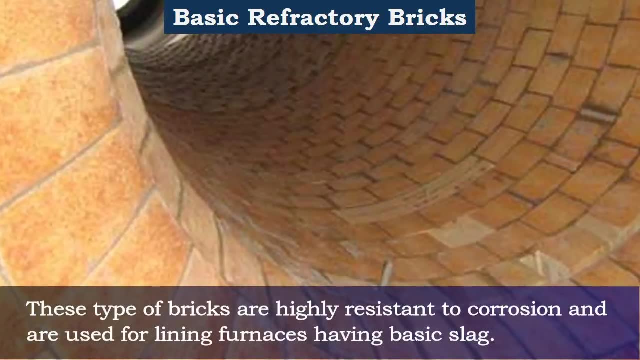 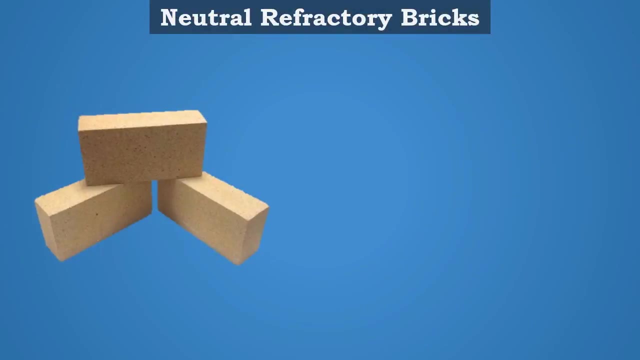 Bauxite bricks consist of aluminium oxide above 85% and clay up to 20%. These type of bricks are highly resistant to corrosion and are used for lining furnaces having basic slag. Neutral refractory bricks. Neutral refractory bricks are available in different varieties, such as chromite bricks, chrome magnesite bricks, spinal bricks and fistrite bricks.